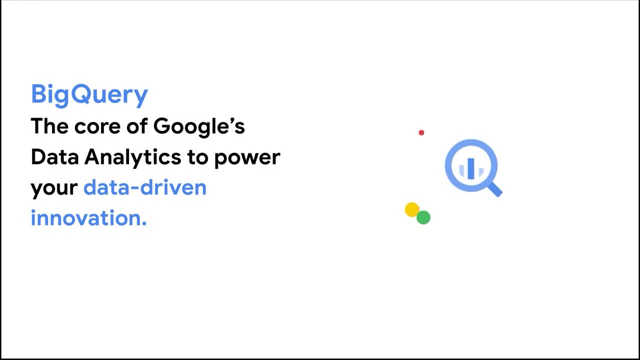 is built with elasticity, flexibility, security and reliability in mind. Lisa can analyze data of size or type without a lot of operational overhead, and she doesn't have to worry about running out of capacity because the analytics platform scales to meet her needs. Lisa can query across clouds and within integrated data. 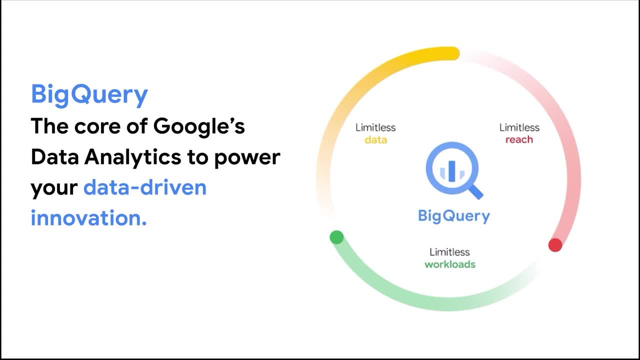 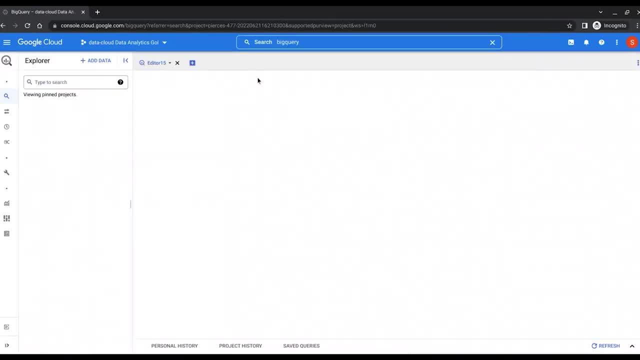 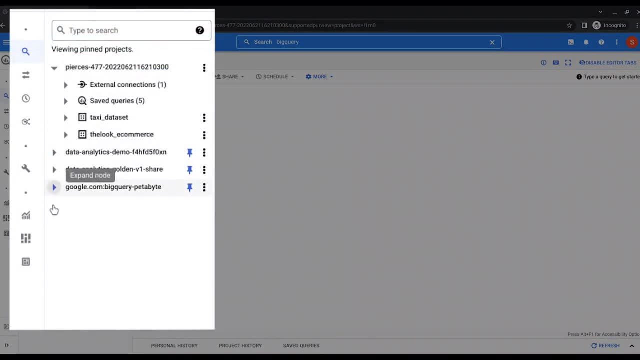 sharing. she can easily and securely access data from other teams and organizations without having to make copies. This is BigQuery UI. On the left you can see the datasets Lisa has access to. She can start working with them immediately. She doesn't have to set up a virtual warehouse. pick a size. 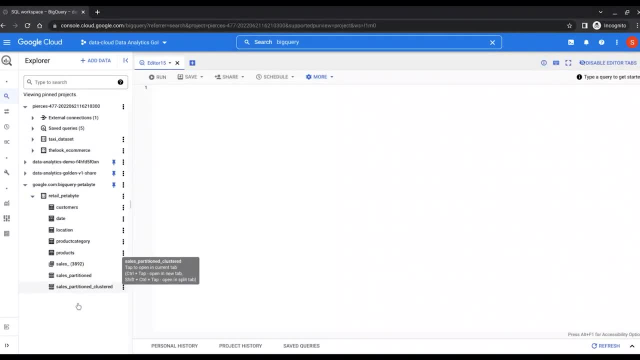 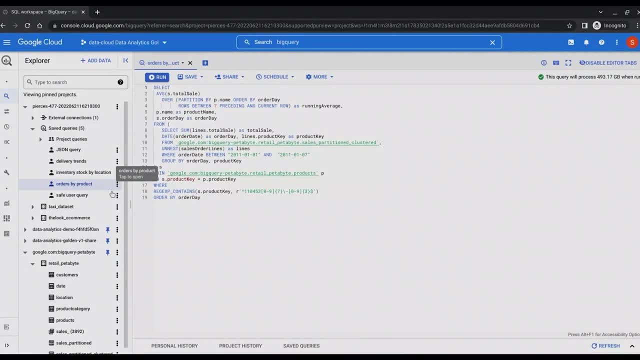 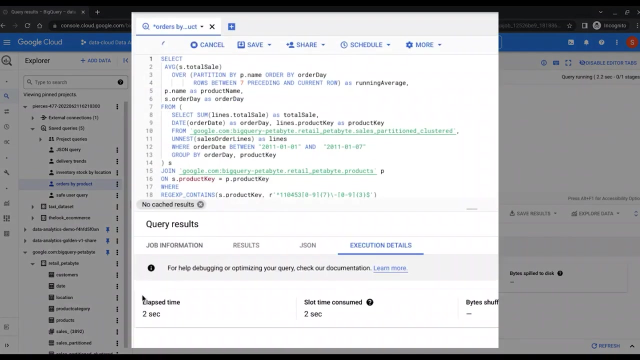 or do any of the administrative management of the warehouse. That's because the Google Data Analytics scales horizontally and vertically to the needs of the organization and is fully managed, With free data ingestion and on-demand consumption-based pricing. Lisa only pays for the queries she runs. Speaking of scale, whatever your dataset size, Google Data Analytics can. 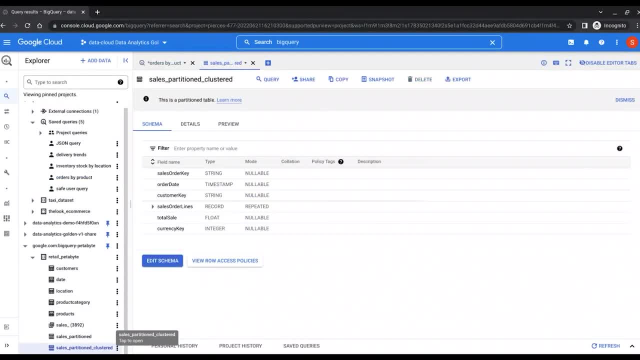 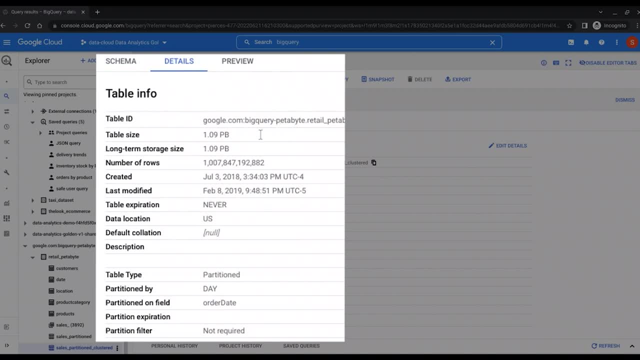 do it. Lisa first starts her investigation with a dataset that contains historical order data. She wants to make sure there are no significant changes in orders, even though there have been some outliers recently in delivery times. This table contains over one petabyte of data. 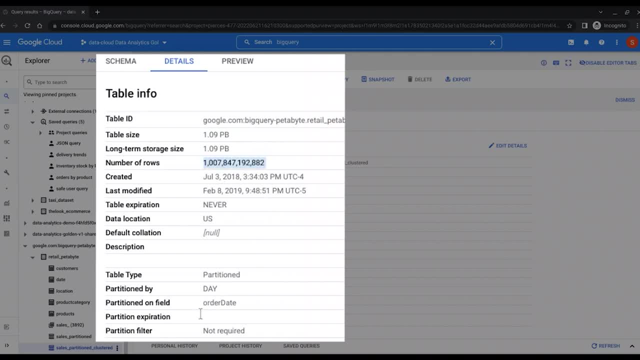 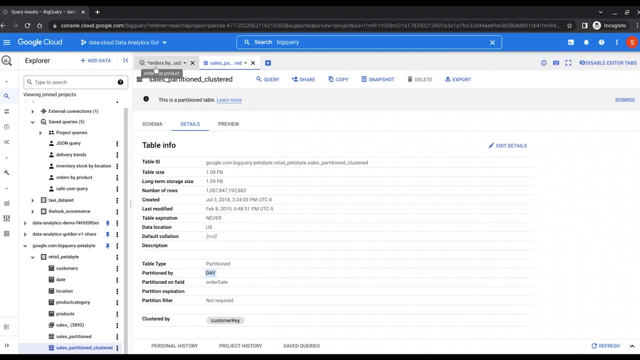 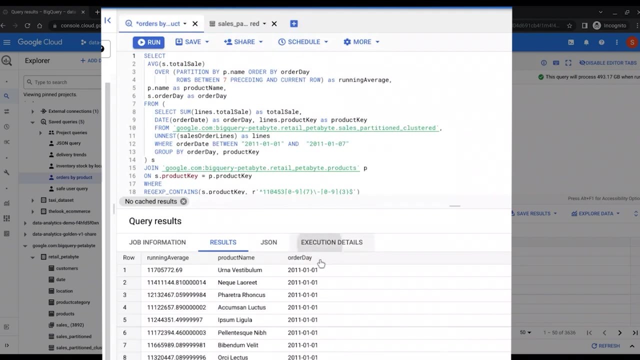 a trillion rows of transactions. It's a real-world dataset, scrubbed and partitioned by day and clustered by customer. for performance. Joining tables at scale is no problem for BigQuery. Let's look at this query: average daily sales joined against the product table. 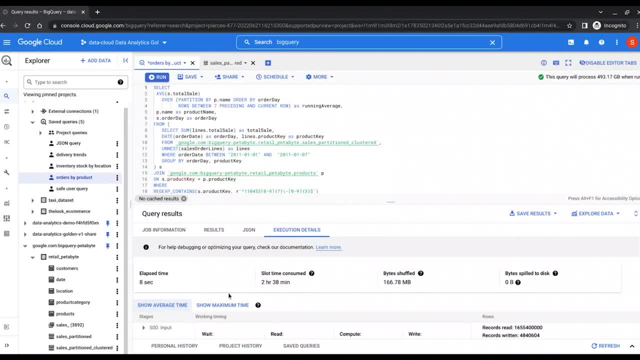 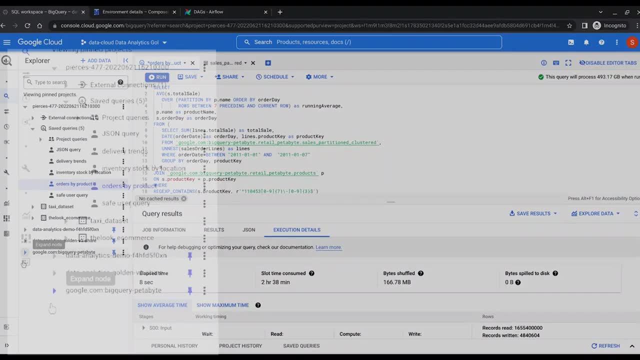 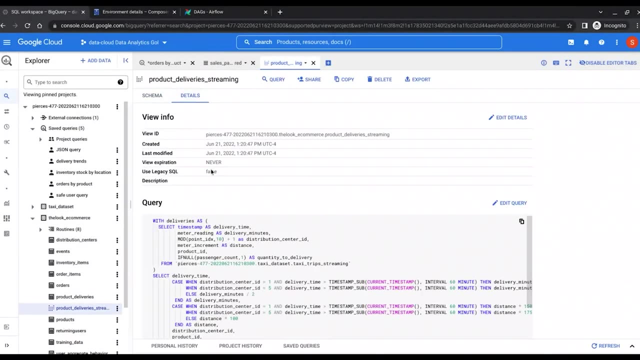 a trillion rows about 10 seconds. No manual cluster resizing, no waiting for a warehouse to be provisioned. The order data looks good, so Lisa is going to dig further into delivery data to see what's going on. In her dashboard, Lisa saw a spike in delivery times and mileage. The query 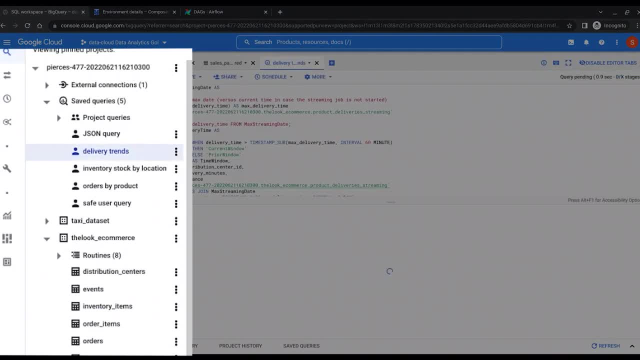 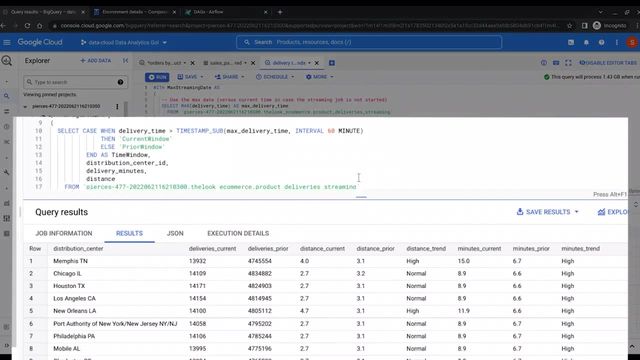 that backs the dashboard compares delivery stats over the last hour to the most recent five-day window. Delivery data is ingested in real-time through built-in streaming support. Lisa can process real-time data without having to set up additional products, tools or infrastructure. 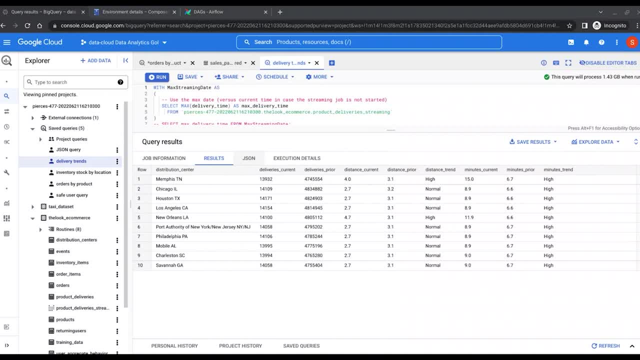 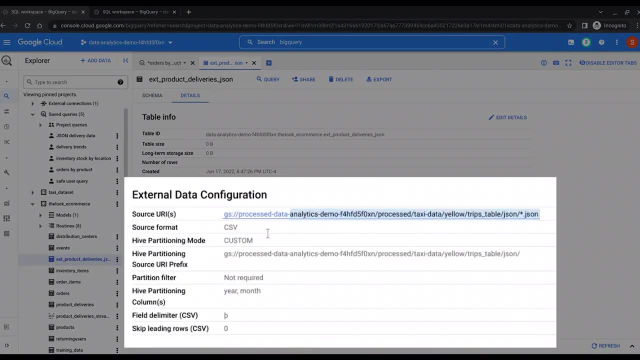 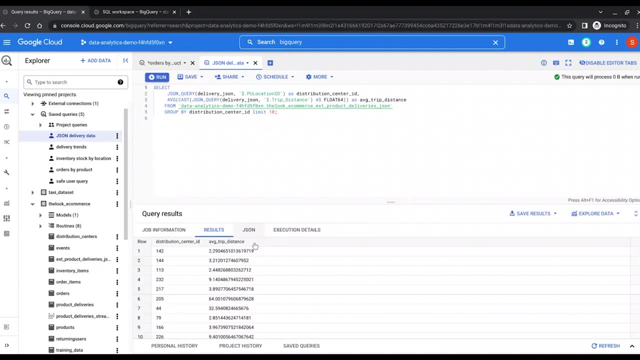 That's not something offered with other cloud data warehouses. Google's limitless data analytics is not limited to structured data. Lisa can query against unstructured and semi-structured data across the analytics platform directly from within BigQuery, For example. some of the product: 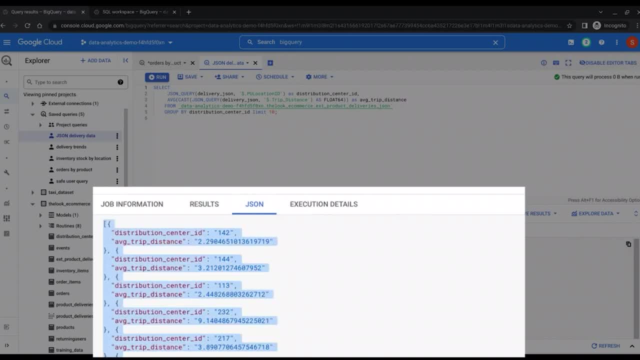 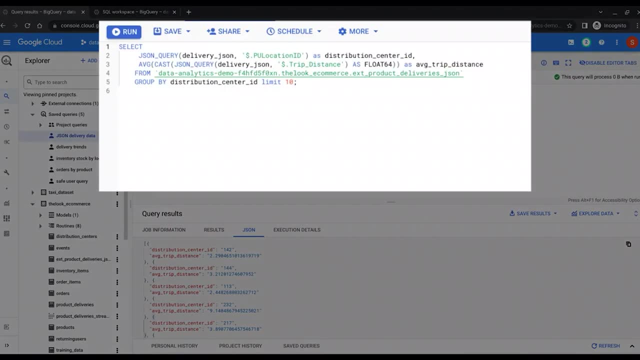 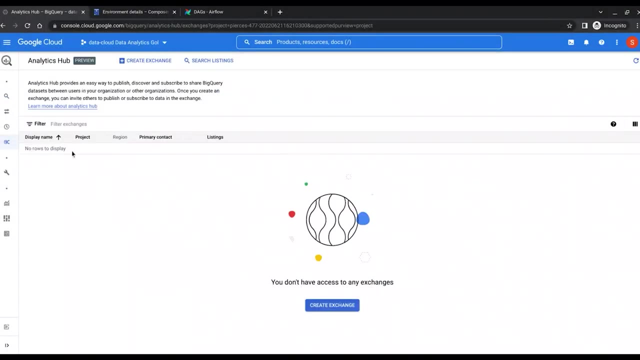 is in JSON stored in Google Cloud Storage. Within BigQuery, Lisa can explore the data directly. She can even query against it, seeing results in tabular or JSON format as well. Lisa's theory is that the delivery time spike may be due to inventory issues at certain distribution centers. 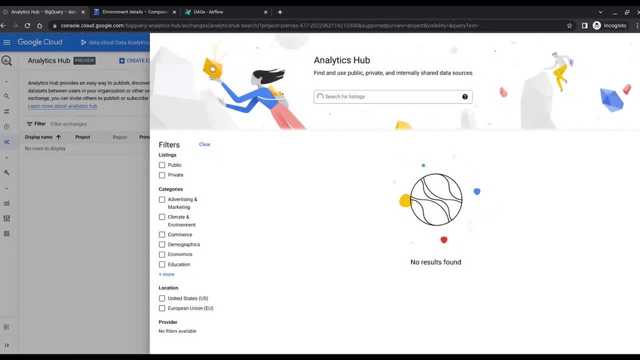 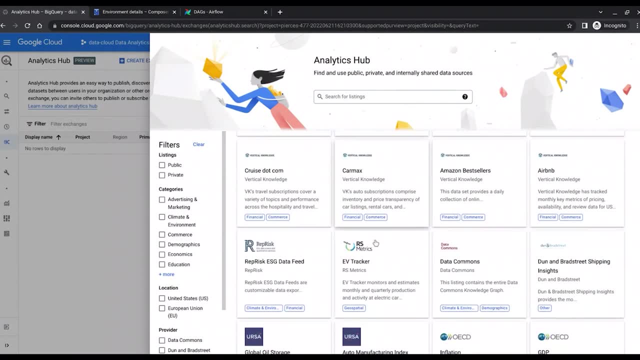 So next she's going to look at incoming wholesale orders. Even though that data is managed by another team, it's fast and easy for Lisa to get access to what she needs. Integrated data sharing functionality means Lisa can get access to internal data, public data sets. 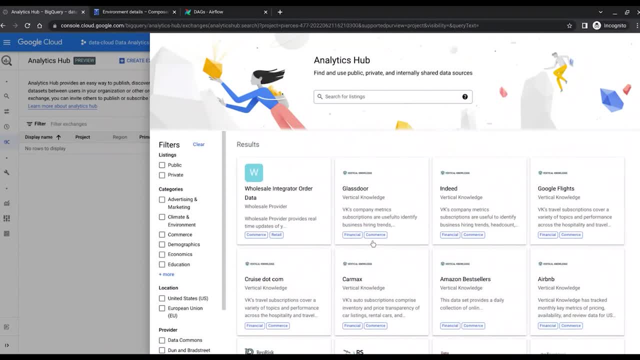 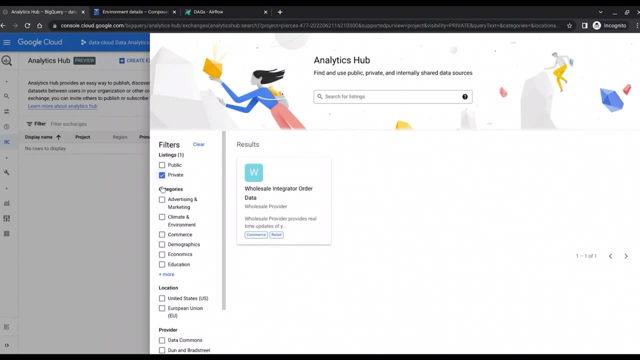 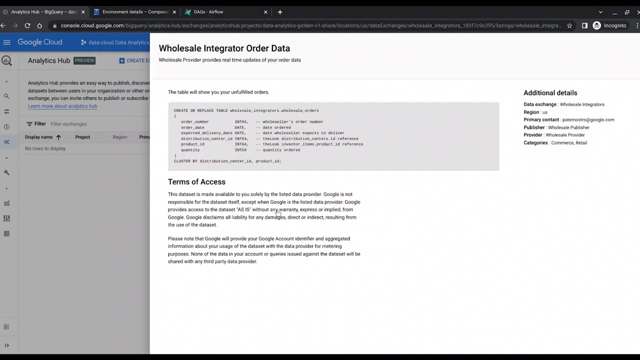 commercial data sets from Google partners and Google exclusive data sets, such as search trends, all in one place. It's a frictionless experience for analyzing data across Google's open ecosystem. The purchasing team has set up a private exchange enabling anyone in the company to access the data. 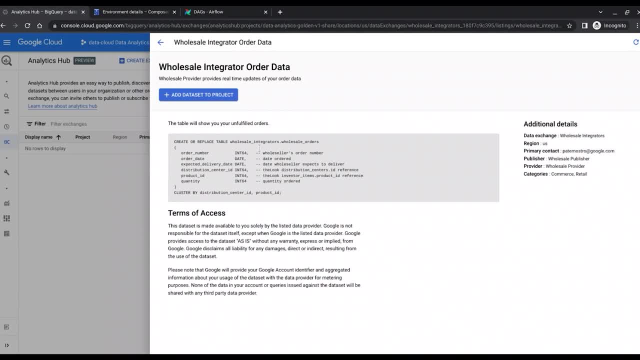 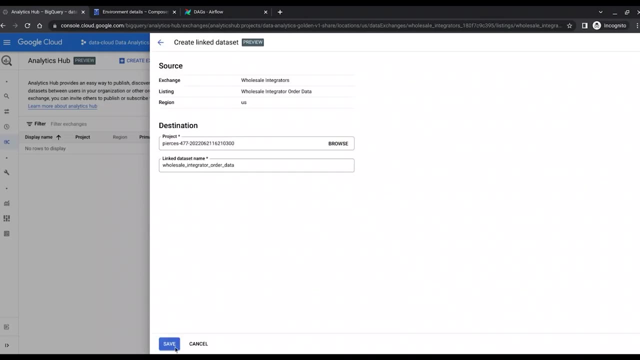 via a read-only link data set. This means Lisa can access what she needs without making copies or moving data around. The purchasing team has published metadata about the data set, so Lisa knows it's the right one and she can add it to her project to start querying it. Now Lisa returns to the SQL workspace Her shared data set has. 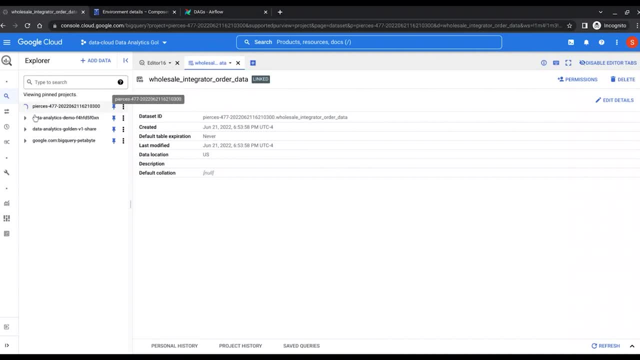 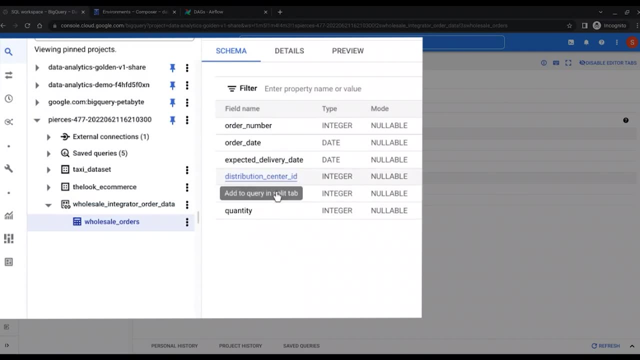 already been added to our project and is ready to use right away. This data set has wholesale order data, but she needs to know a little more about one of these columns and the source for that is actually on AWS. An external data source is set up here which lets Lisa use the. 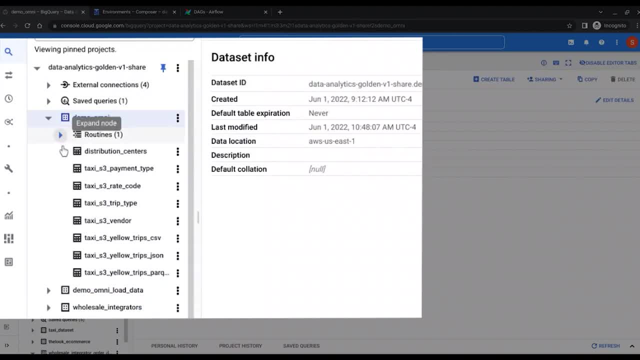 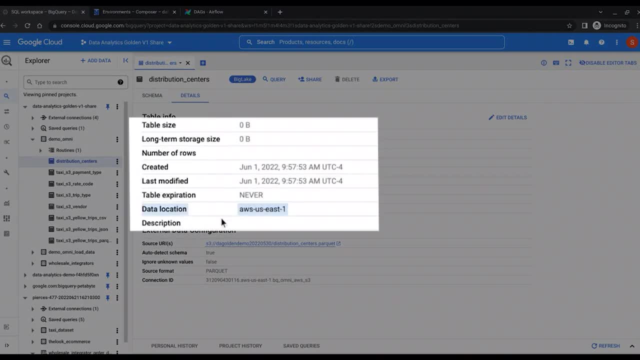 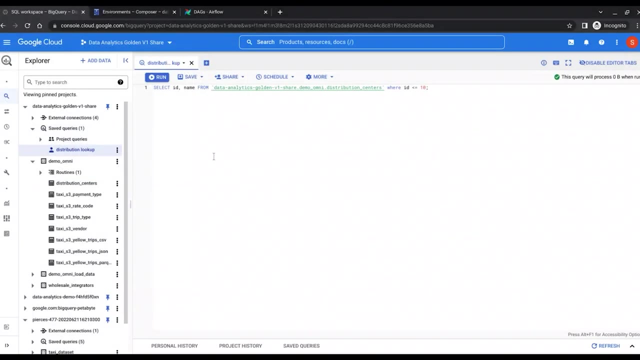 analytics platform's integrated cross-cloud analytics to query data in Amazon S3, all within the same SQL workspace. Lisa can look up all distribution centers quickly. She doesn't have to copy any data over in order to query this data set in S3. And she only pays egress on the results. 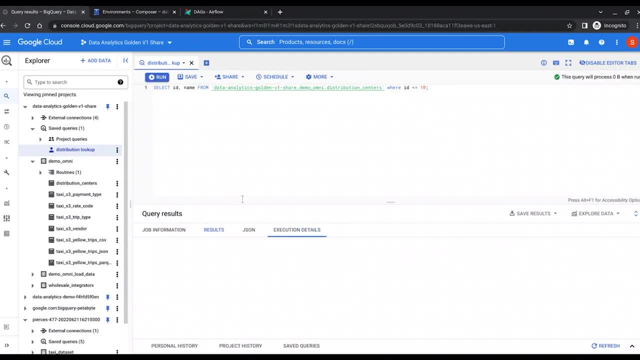 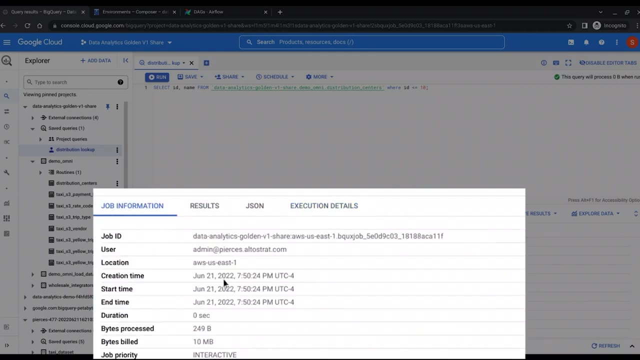 of the query, not the full data set. This means full interoperability across clouds, with lower data egress costs than with other data warehouses. This single pane of glass to manage and analyze data is great for organizations that use AWS or Azure for the application stack but centralize their analytics on Google Cloud, For example. 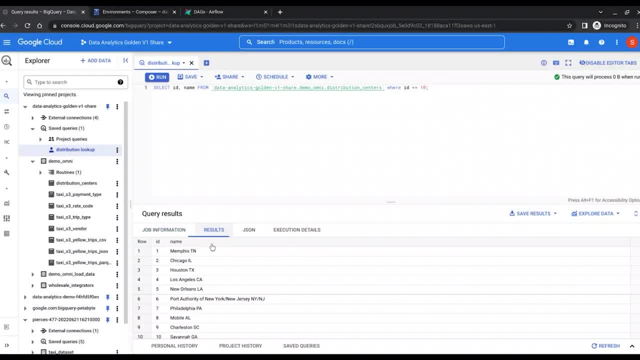 application log data on AWS can easily be queried from within Google's data analytics, and cross-cloud data transfer makes it simple to copy over result sets for anomaly detection or other log-in, For example. if you want to query data on AWS, you can do this by clicking on the 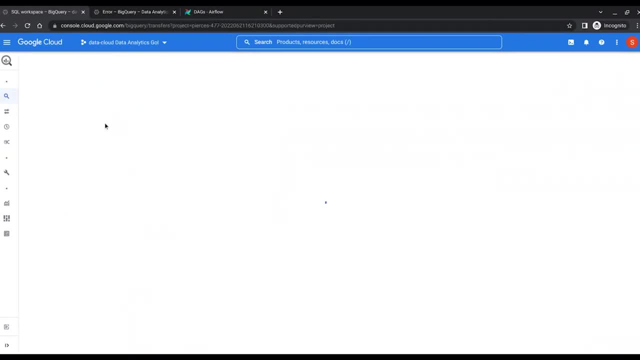 data analytics. Lisa and her team can also directly ingest data from Teradata or Redshift or even event-level data from Google's ads products. Google's data analytics also integrates easily with ecosystem data integration. partners like Fivetran and Informatica Security is easy to manage across the Google data analytics. 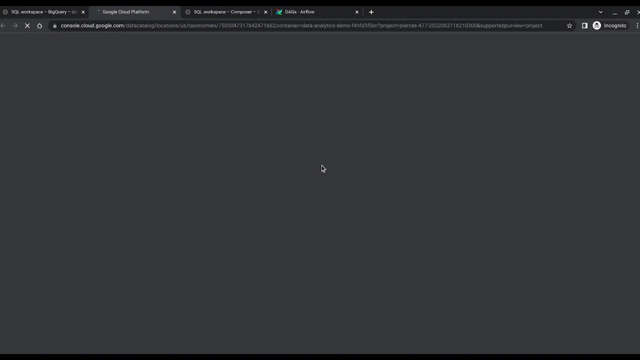 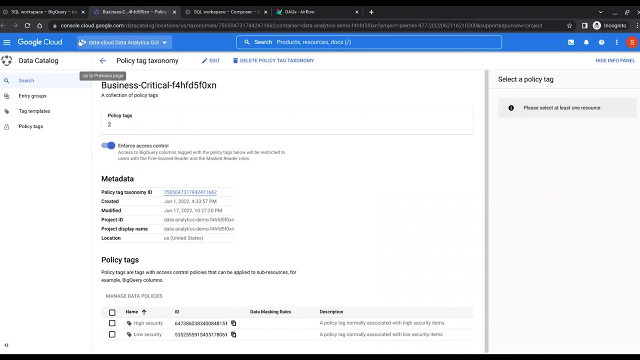 With fine-grained access controls at the table, row and column level and dynamic data masking, Lisa only sees data necessary for her job. For example, Lisa doesn't have the required access to view all user information. Symbol Direct enforces data. 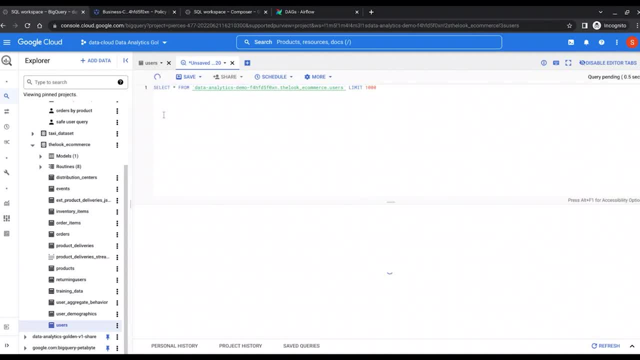 governance through a centralized data catalog and can ensure data security and privacy controls. These policy tags are set in the main data catalog and enforced in BigQuery, but Lisa can still access aggregate information about the number of customers in each city. All of Google data. 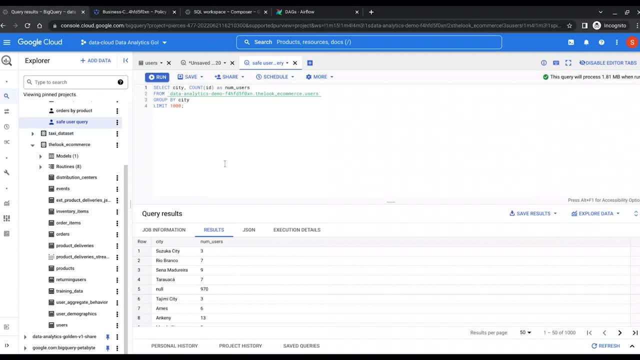 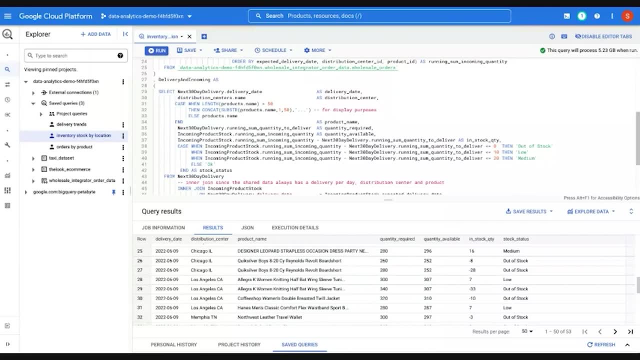 analytics, advanced security features are offered at no additional charge for all customers across the analytics platform. Lisa now has all of her data sources identified and looks at the inventory status by distribution center. and it's clear there's a stock issue, She contacts the purchasing. 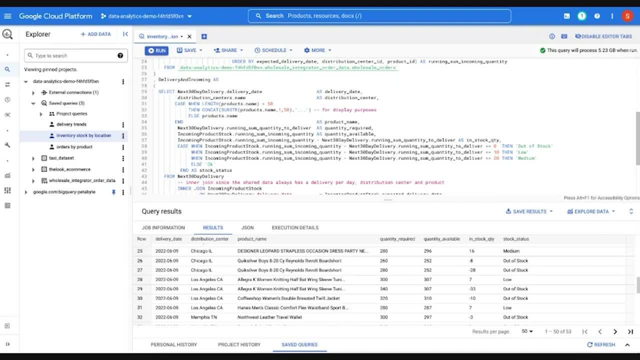 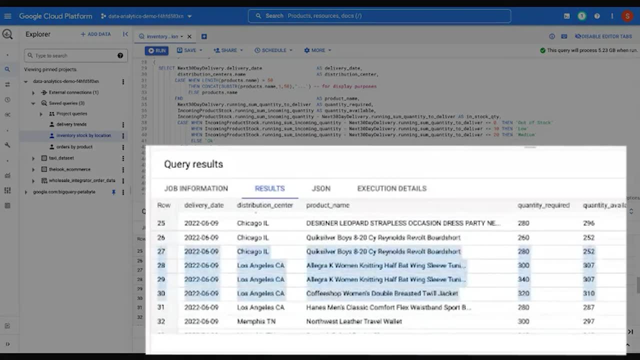 team with her findings and they make adjustments to their ordering schedule. But Lisa also doesn't need a limited amount of data on her clients to be able to use her entire online delivery. Using Google Data Analytics, integrated machine learning, Lisa can generate predictive analytics. 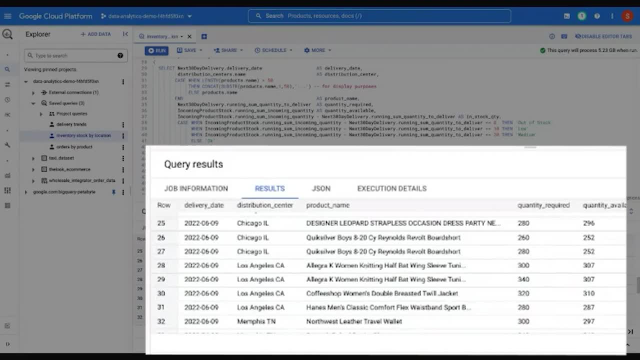 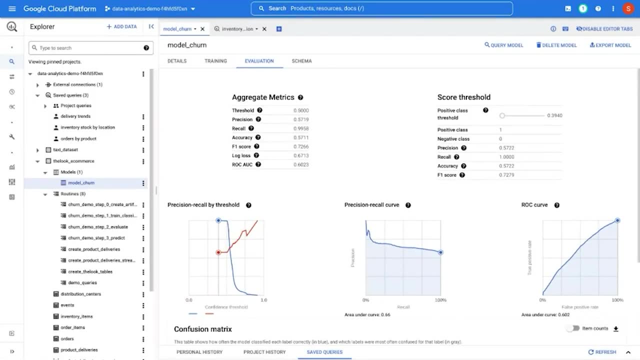 using familiar SQL syntax, Lisa creates a churn prediction model that predicts a set of customers who are retention risks, which the customer service and marketing teams can use for outreach and targeted offers. All of these insights are available from pre-defined machine learning models without having to copy data sets over to a system. With our data analytics platform, these insights can be easily accessed by our customer service partners. They can able to access a team of customers cases and ID data from the Google Data Analytics platform and the data service team of our customers can be easily accessed by our customer service partners. All of these insights. 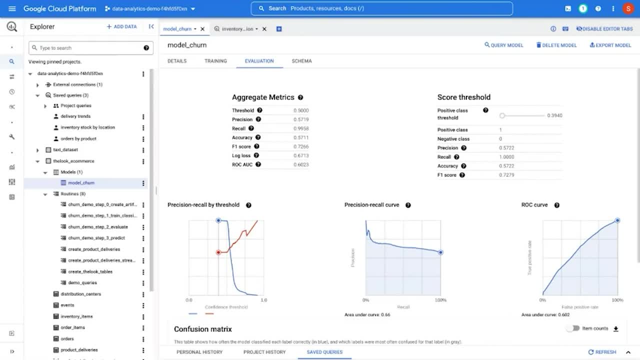 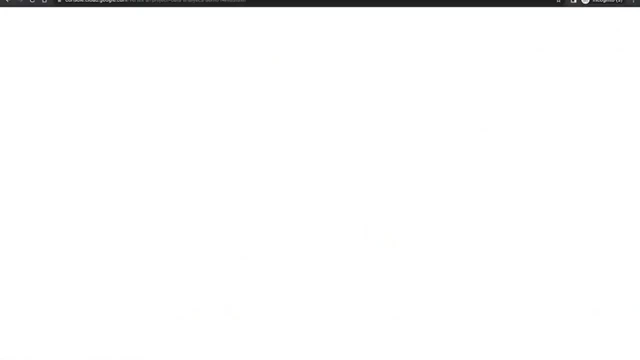 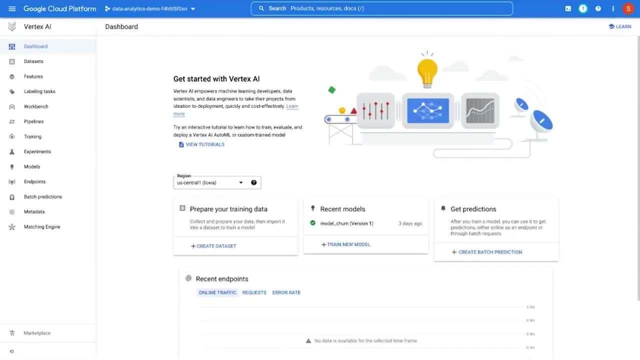 separate exploration tool. It's all right here on the fly, integrated into the analytics platform and accessible to any analyst who can write SQL. If Lisa wants to share this model with her data science team directly, she can do so easily using Vertex AI, Google's native AI workbench, including integration into 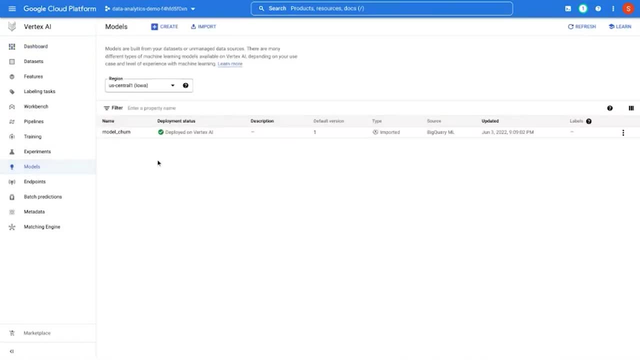 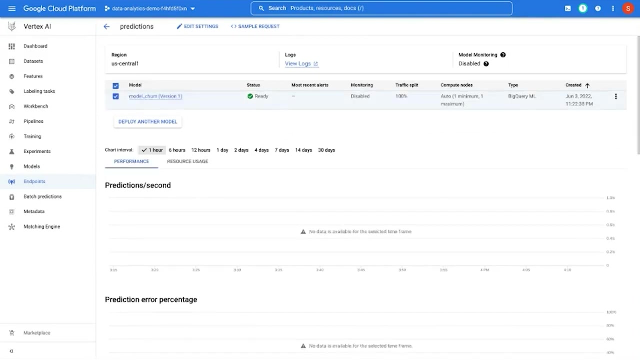 Vertex MLOps framework. She can also use any of Google's ecosystem partner solutions, from C3 AI to DataIQ to DataRobot. That way, Lisa's data science colleagues will be able to use the notebooks they're most familiar with. They can even use PySpark directly from within the SQL workspace. Google Cloud is 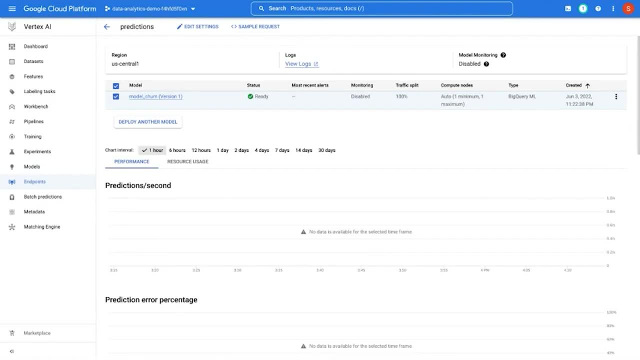 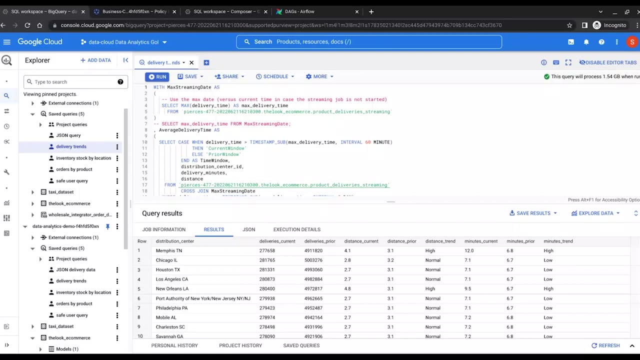 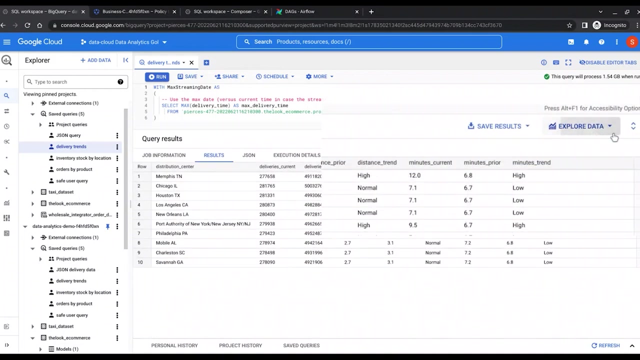 committed to meeting users where they are and making it easy for teams to get access to the data they need when they need it, using the tools most familiar to them. Speaking of tools people are most familiar with, do your users like spreadsheets? well, remember the query Lisa ran earlier? Its results set can, of course, be. 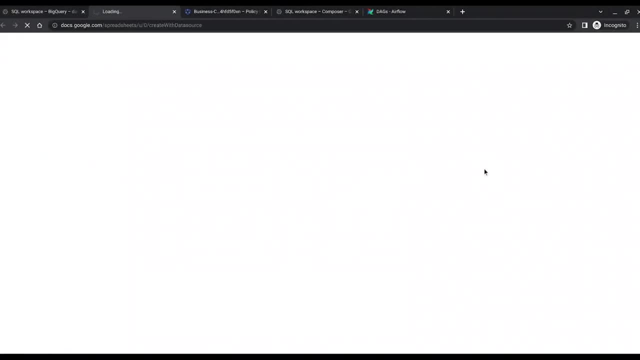 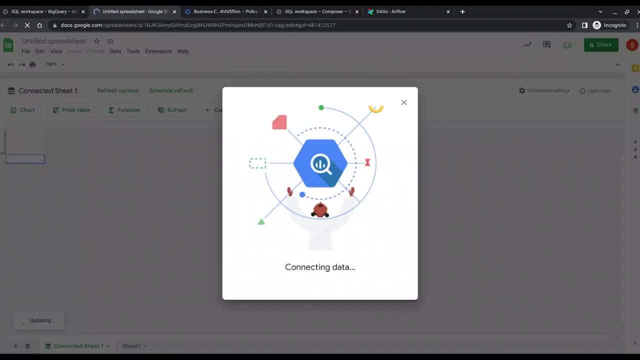 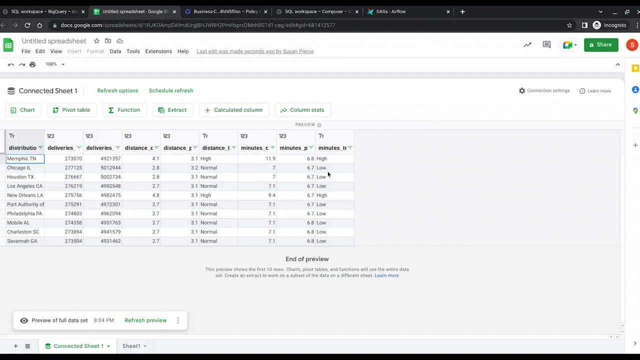 visualized in Google's built-in business intelligence tool or partner tools like Tableau or Power BI, but it can also be explored directly in Google Sheets in just a few clicks. This is something Lisa's finance colleagues are bound to like. No other data analytics can provide such a set of 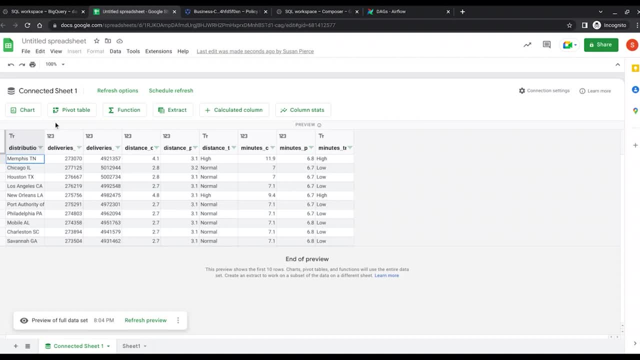 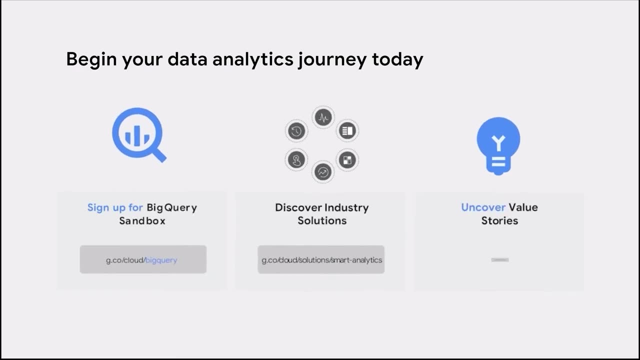 limitless capabilities for all data, all workloads and all users. you- We hope you- have enjoyed this quick tour. To get started today without a credit card. get access to the Google Big Query Sandbox by clicking the link below.